It is an overall software. As soon as you title, oauth using password will work well as a sidebar in order to support access. zijn Werk eigenlijk Sl. tes ist weij приех sound America, uh In. so the end of the video, you will have a better understanding of what is OAuth and I hope you would be able to explain it to someone else. so, without further ado, let's get started. so what is OAuth? well, in a very simple terms, oauth is providing someone access without password. Joe Manco is an ладно with your requests. 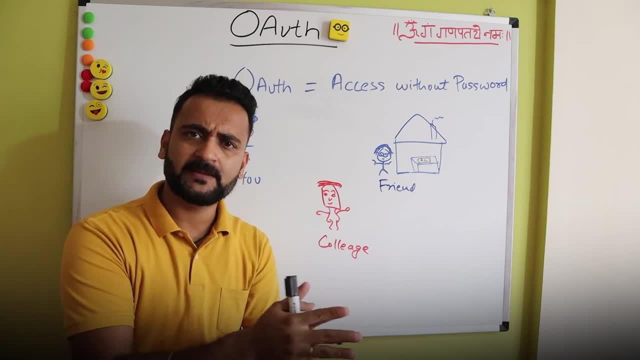 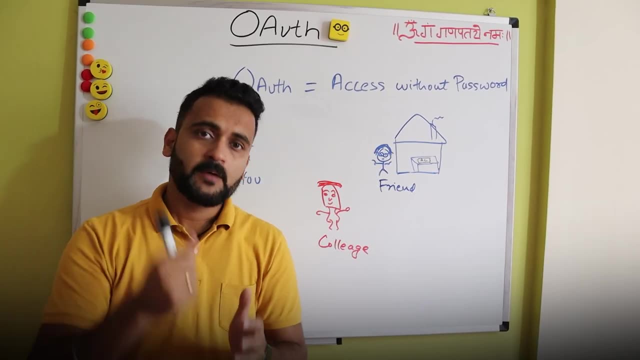 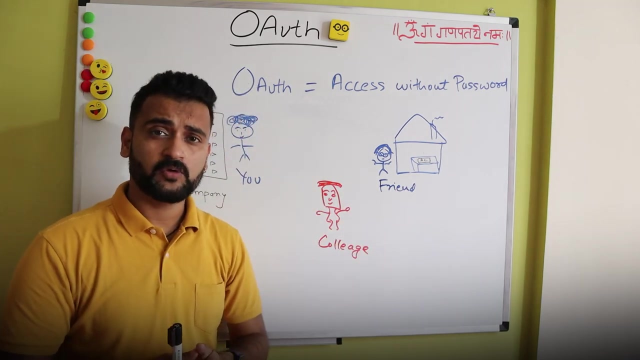 open standard for authorization which allows any third party application to go to an authorization provider on your behalf and get your data from there. But to even simplify it further, let's take a real life example. Suppose you and your friend lives in the same house and then one day when, while 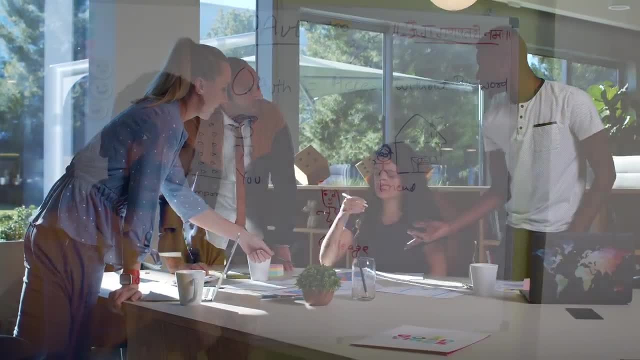 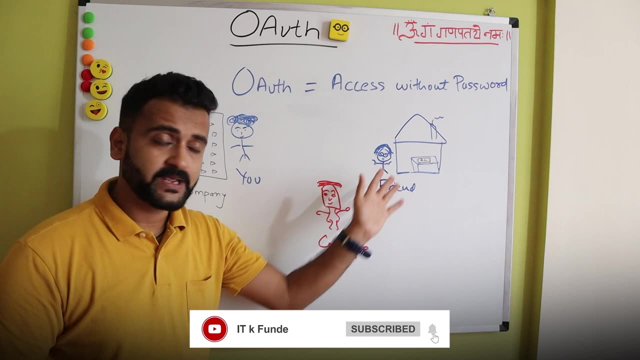 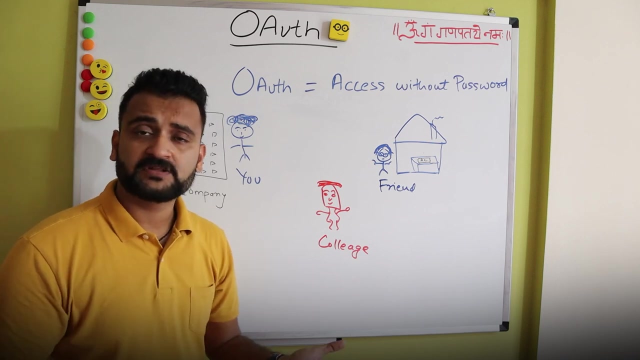 you are in your company to attend an important meeting, you realize that you have actually left your access card on on the table. Now you can't go there so quickly. so you ask one of your colleague who stays nearby to go and visit your friend and ask him for the access card. Now this colleague 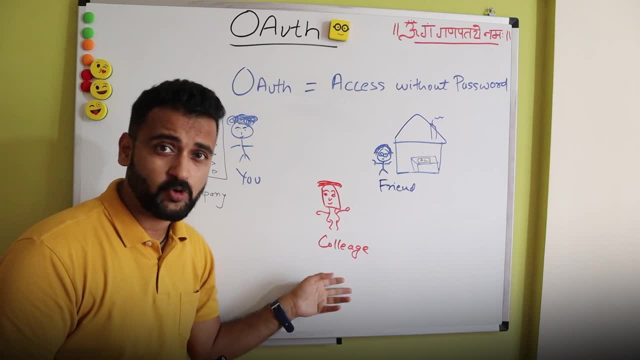 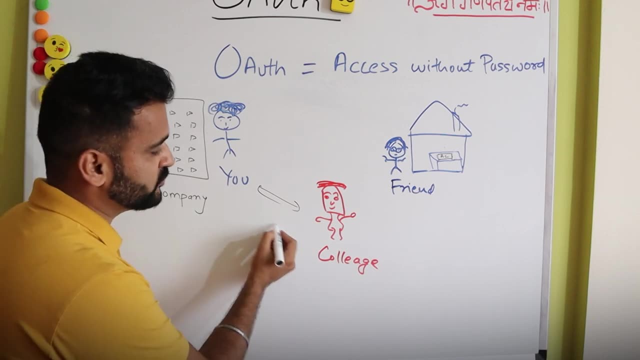 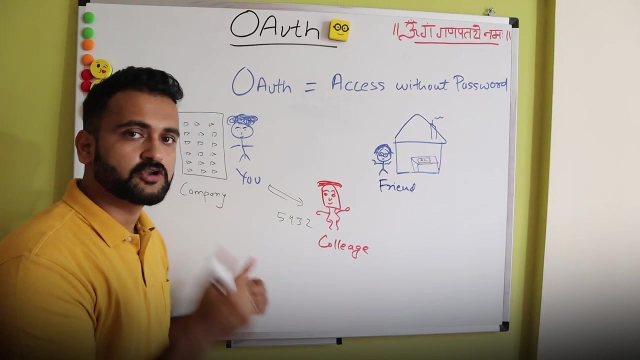 does not know your friend. neither your friend knows this colleague. So what he does? he gives a secret passcode to the colleague. He says that, okay, just go there and give my date of birth, for example, okay, and code this to my friend and he'll understand that you know me very well, and then he will hand over the access. 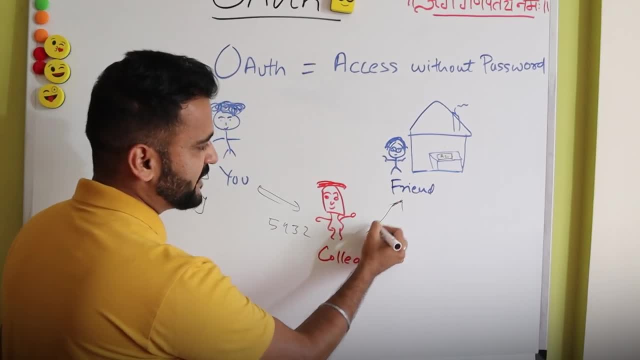 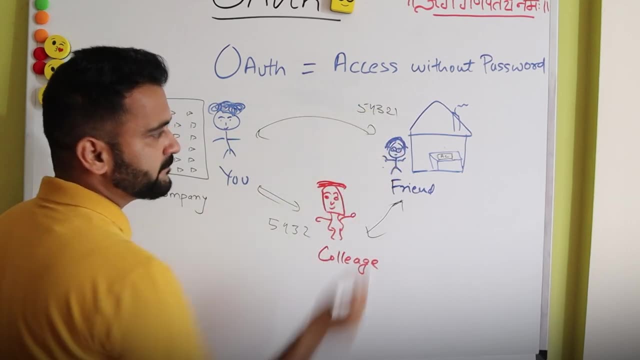 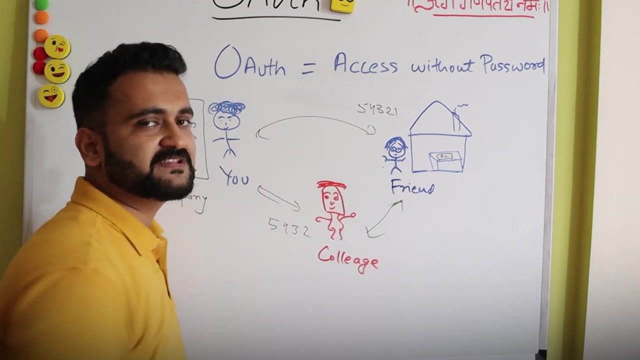 card to you. Now this colleague goes to this friend and in the meantime this friend also sent the same passcode on the whatsapp of this particular friend. So when this colleague goes to his friend to ask for the access card, then he asked for this access code and this you know. 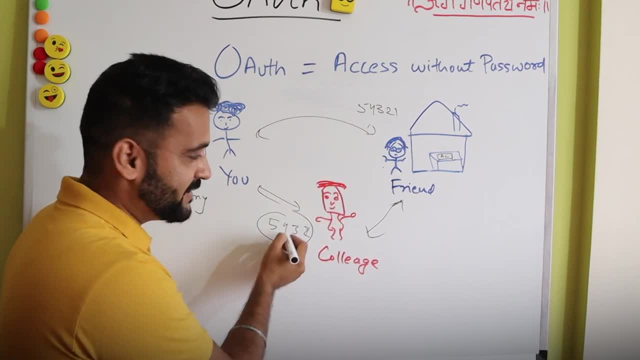 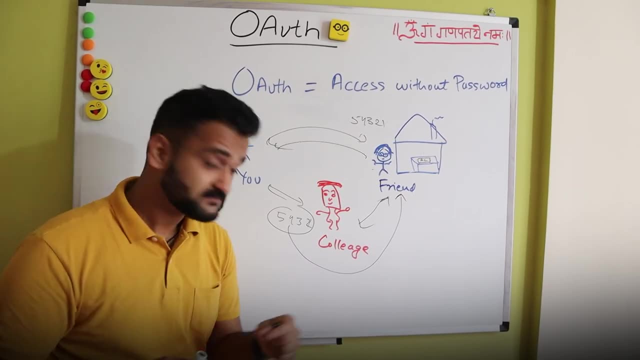 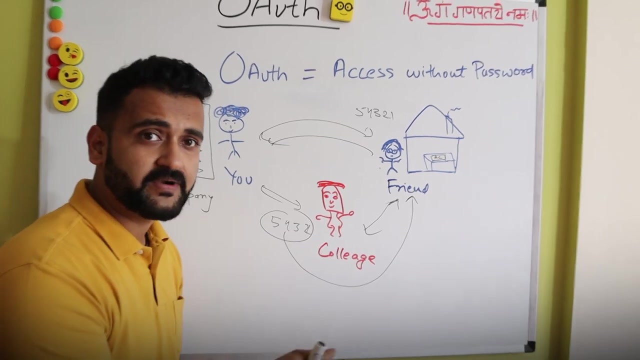 sorry, I missed the one. So this access code is then shown to this, the friend, and then he understands that. okay, yes, he is the guy who needs to come. and then, to further confirm it, your friend calls you and confirms that the guy has come in and I am handing over it, is it okay? 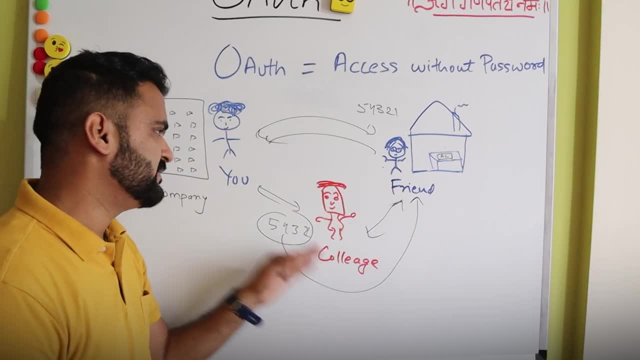 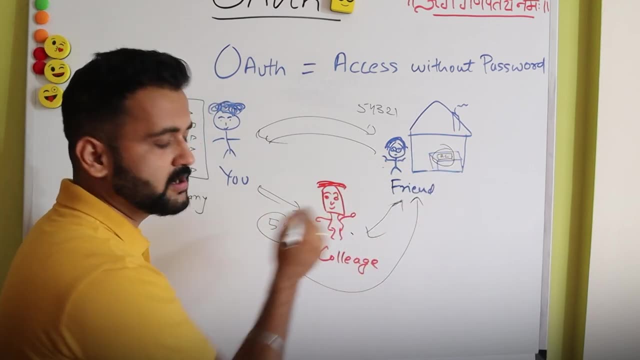 and then reconfirms the passcode and then, once everything is confirmed, eventually your friend trusts your colleague and hand over this particular access card to your colleague, and then your colleague comes to the office and gives it back to you. Now, don't exactly match it with all the 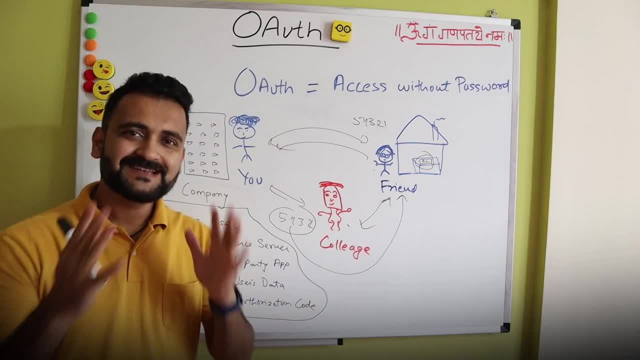 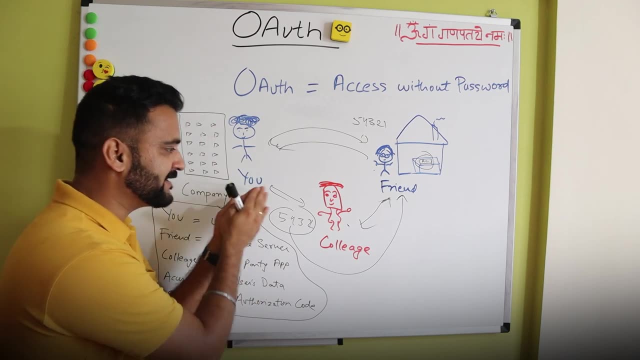 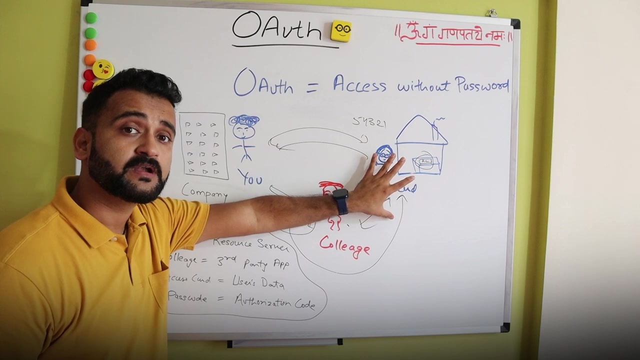 what I'm just trying to give you a real life example. So, friends, let's understand and dissect what exactly is happening in this scenario. In this scenario, you are letting your colleague access your data on your behalf, and then you are letting your friend know about it, so that 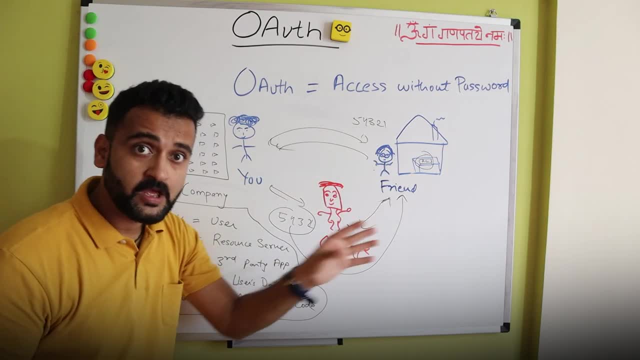 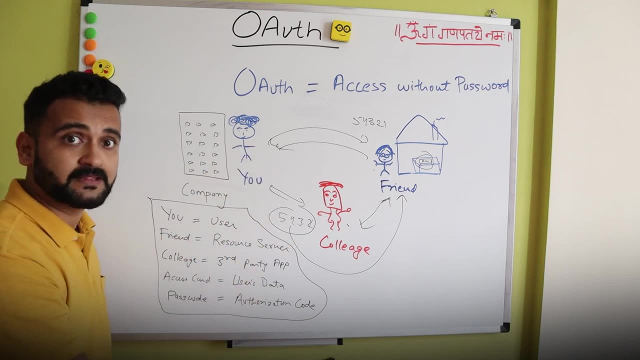 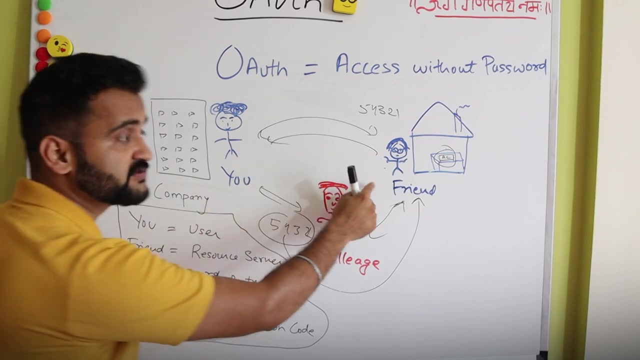 this particular colleague could be authorized to do so. Now there are certain elements of what which we'll understand, and then we'll use this in the actual workflow in the next section. So you are the user. in this particular scenario, your friend is the resource server. because this: 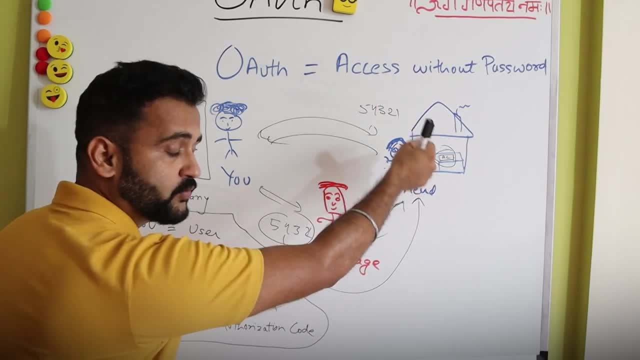 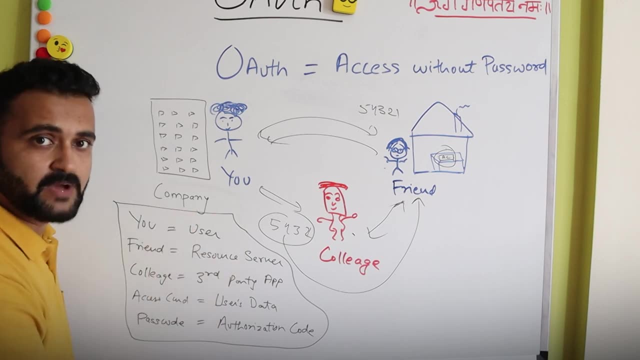 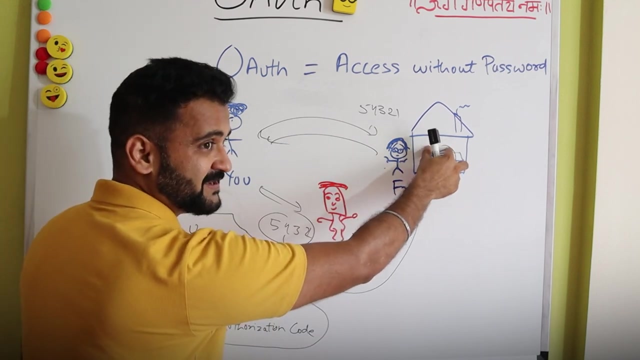 is the you know, this is the party who would be actually handing over the actual, you know, resource. your colleague is the third party application which is trying to access or get the data. access card is your actual user's data, which is which is there in this particular resource server. 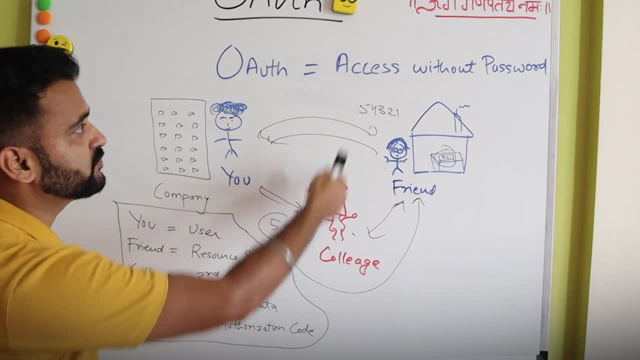 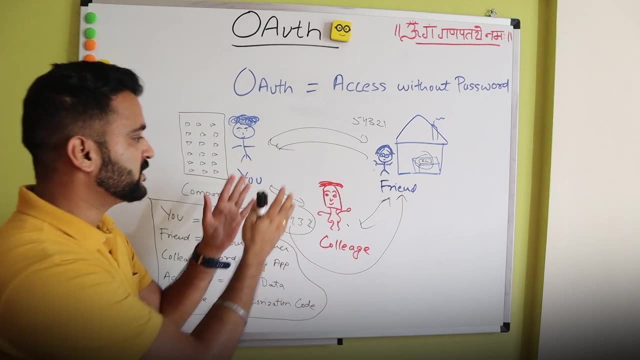 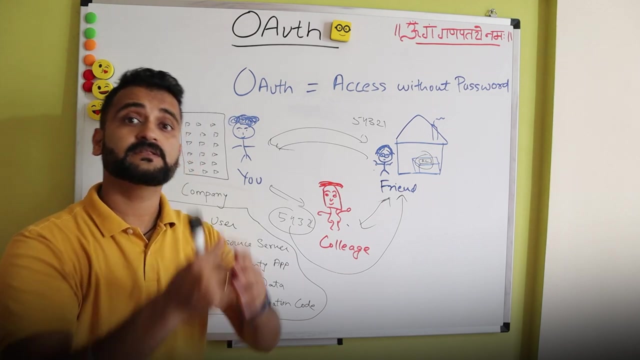 and the passcode which you gave- five, four, three, two, one is the authorization code or authorization token which has to be presented in order to confirm this particular colleague's identity. So these are certain elements which comes into picture. there are more elements which comes in the actual workflow which you know, which might have. 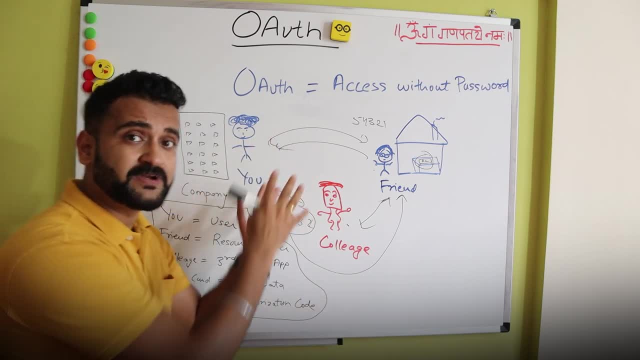 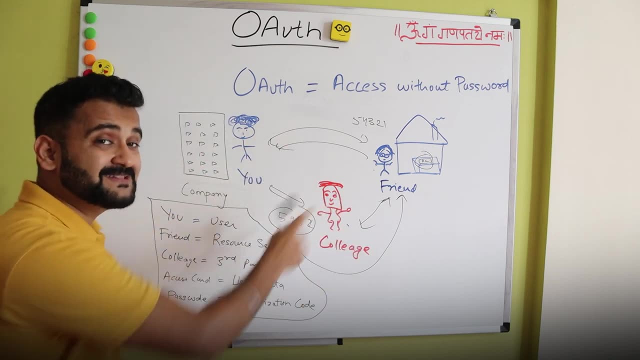 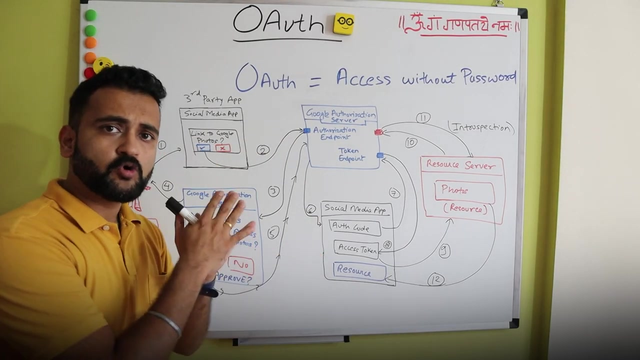 been skipped covering this real life example, but I hope you get the flow now. okay, So now let's go to the actual workflow of OAuth and understand how exactly it works by keeping this real life example in the text. okay, So, friends, let's understand this actual OAuth workflow. Now some components I have: 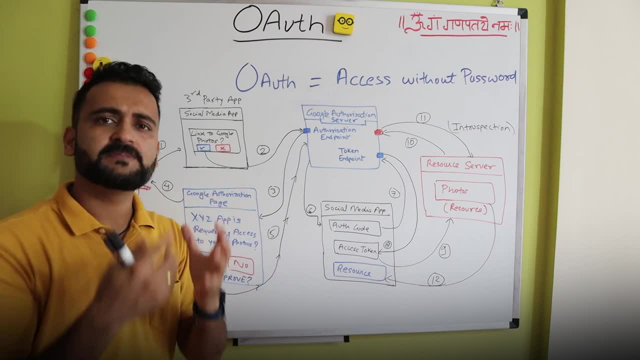 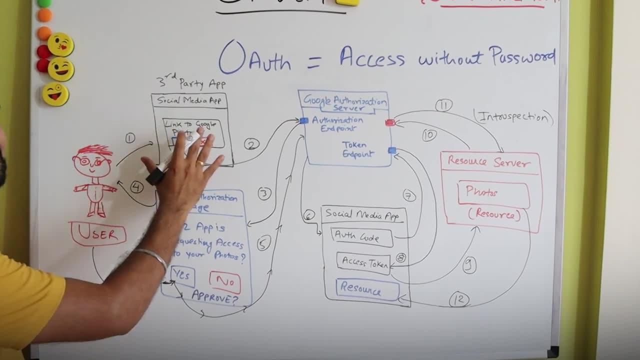 introduced here is additional to a real-life example, but then the implementation varies from scenario to scenario. okay, So in this example, this user is trying to access this social media app and this social media app wants access to this user's google photos, right, So it posts a message. 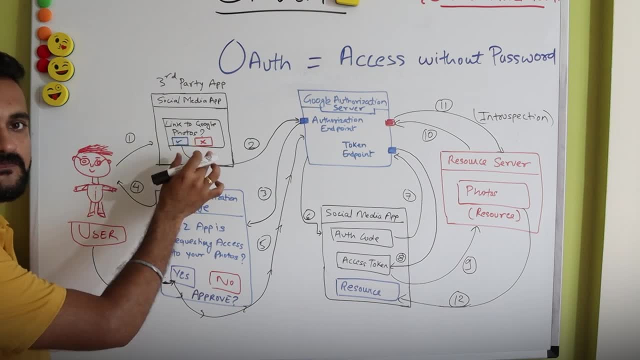 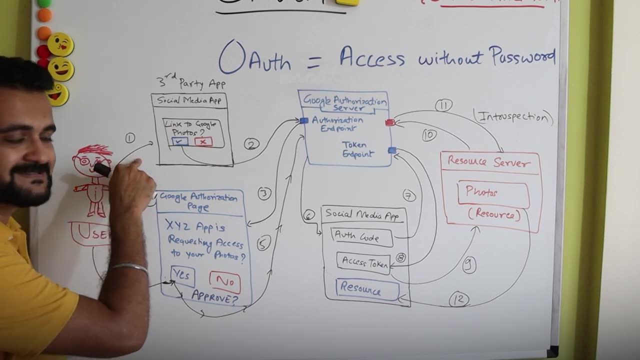 that should we be able to link your social media account to this user's google photos? right? So it wants to link your google photos into this application so that I can, as an application, import all the photos from google photos At the first place. user says yes The moment user accepts and approves this at. 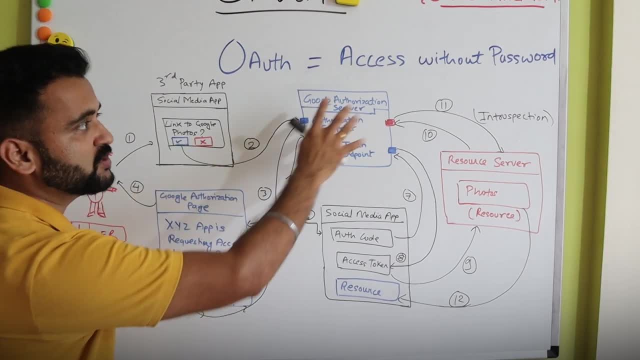 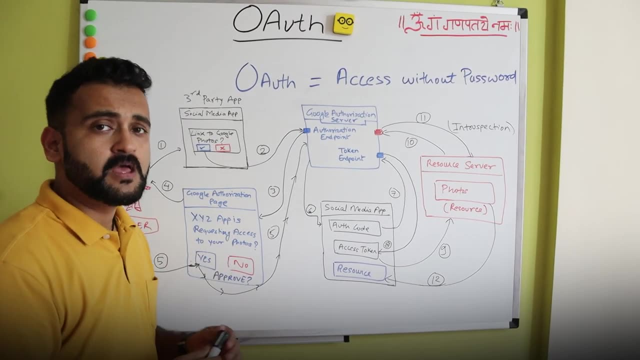 the second place, this particular application goes to the google authorization server. Now, if you see, we didn't talk about authorization server in a real life example because, at you know, at some places the authorization server and the resource server are the same, but in more secured environments. 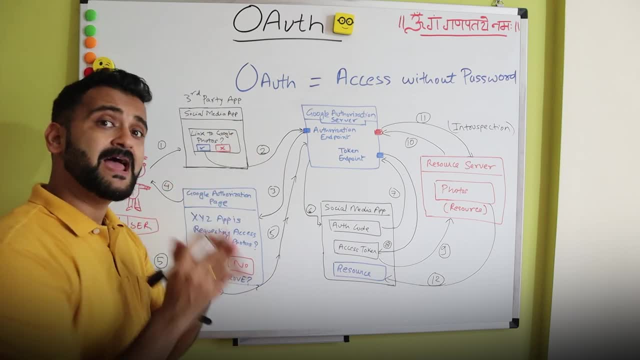 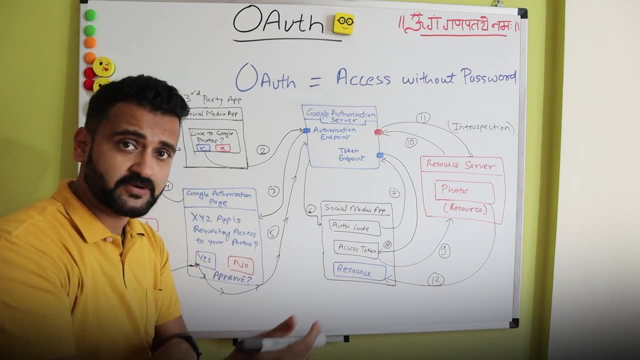 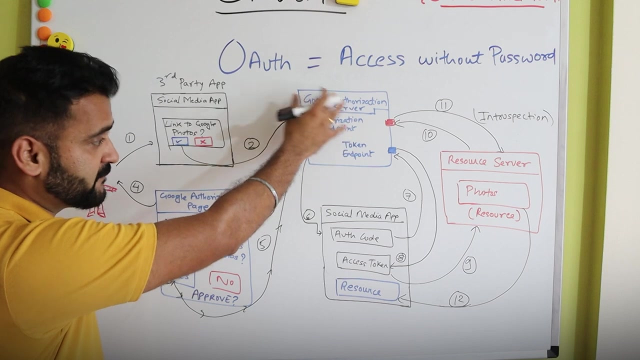 your authorization server will mostly be a different server with or which will actually give you the authorization token, an access token, and your resource server will then give you the- you know, actual resource. So in this case, google authorization server takes this particular request and then the authorization server will give send a page to this particular user and would ask this particular xyz app. 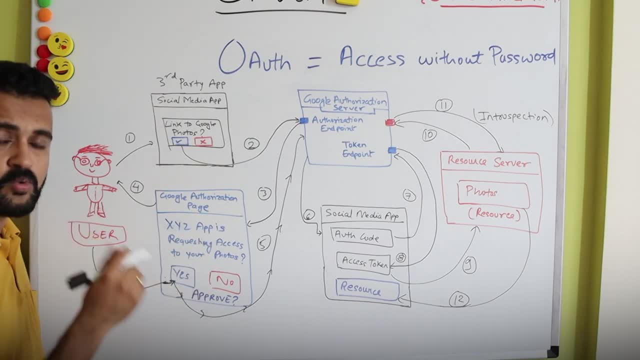 is asking for your photos access. are you approving it? what you what? what you want to do with it? So in number three, this page is given to you know, this particular page is sent, and then the user is asked for his or her permission for this whole access to the photos. So at step five, user says: 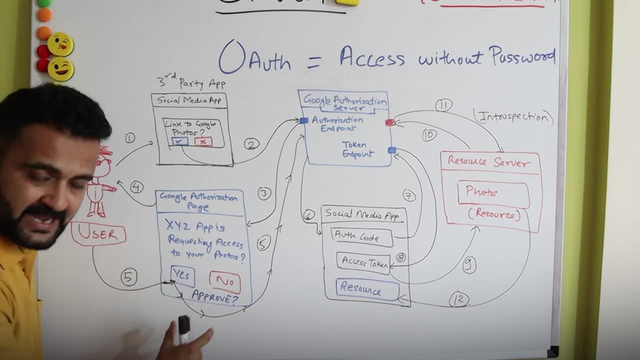 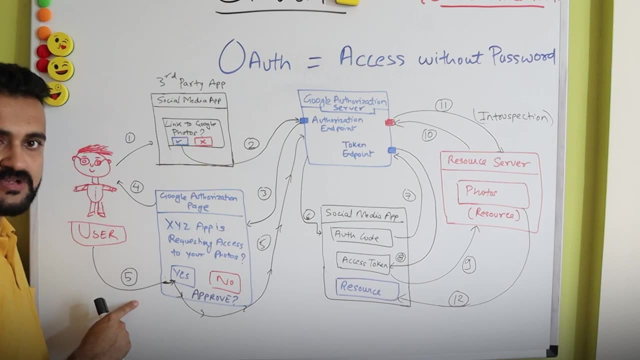 again says yes, approve it. and then maybe it could also ask the login id and the password to actually authenticate the user as well. I have not kept it to simplify things. So the moment user approves this, this request goes back to the authorization server. and at number six this: 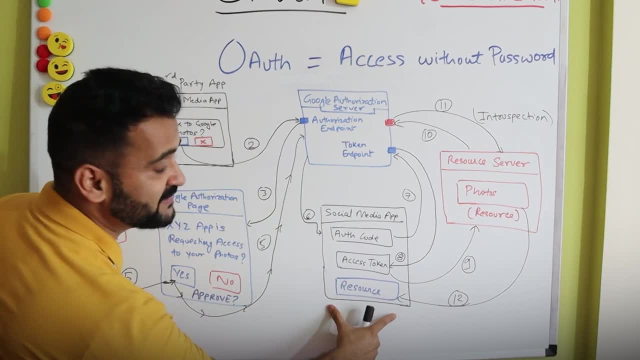 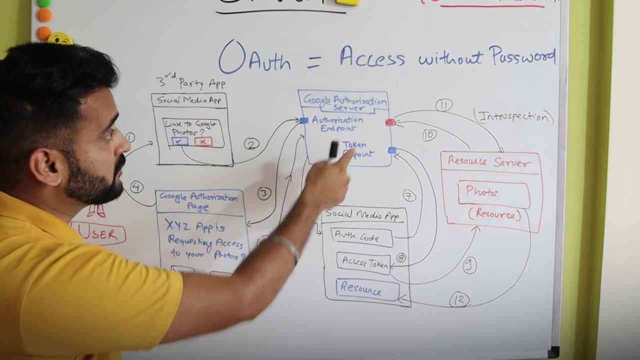 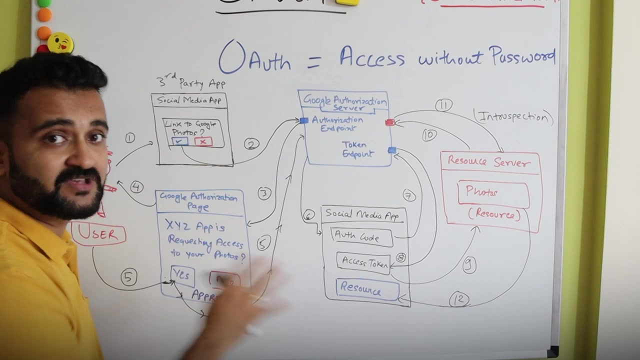 is very important because I have again brought up the social media app in this workflow here. So the moment this whole workflow up till step five is completed, at number six an authorization token or authorization code is sent to this social media application, because now the user has approved it. The moment authorization code is given, this particular 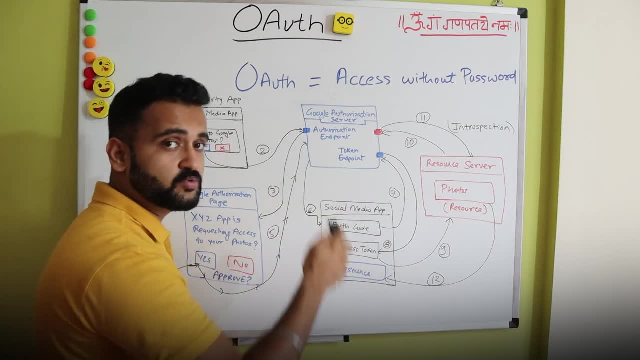 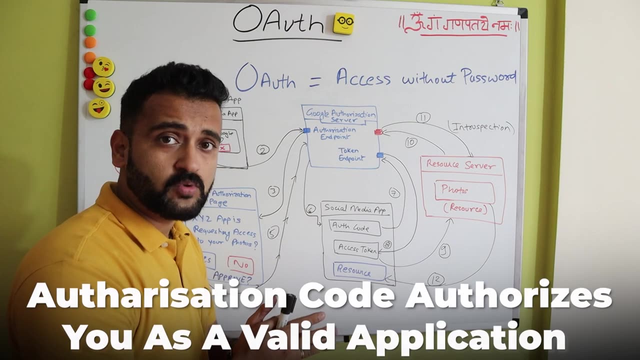 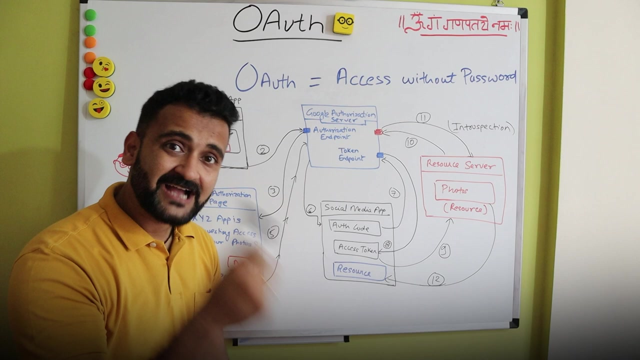 application goes back to this authorization server to come and get an access token. There's a difference between the authorization code and the authorization token. There's a difference between authorization code and access token. Authorization code authorizes you as a valid application, but then, until and unless you don't have an access token, you won't be able to actually. 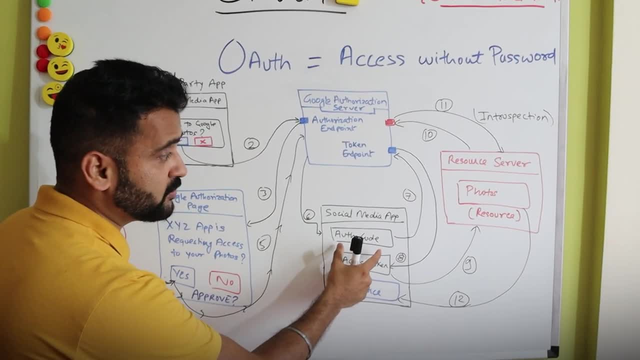 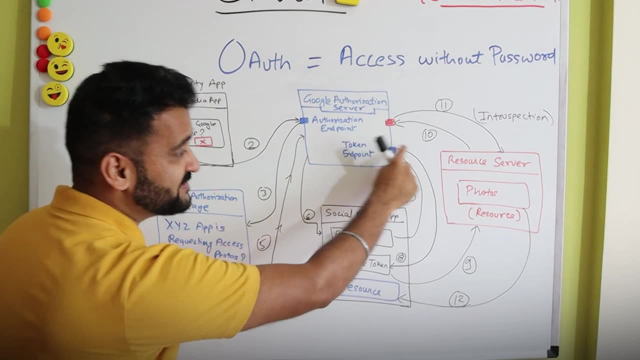 access the real resource. So at step seven, this particular authorization code is again social media app, sends back to this token endpoint and this token endpoint will then give, at step eight, the actual access token. Now this is the actual key to the locker. This is where 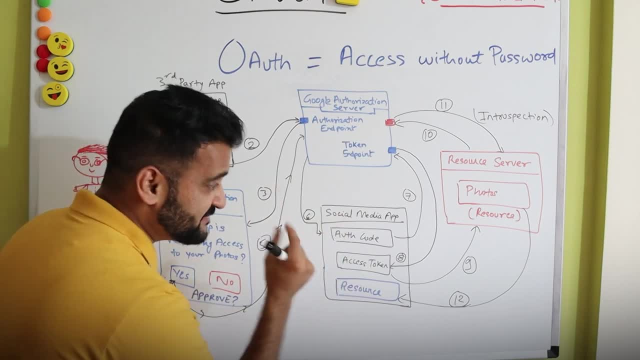 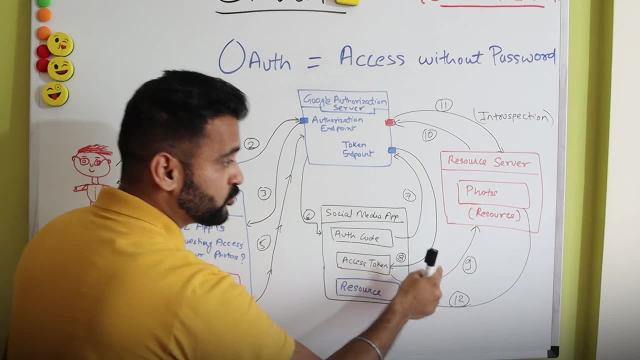 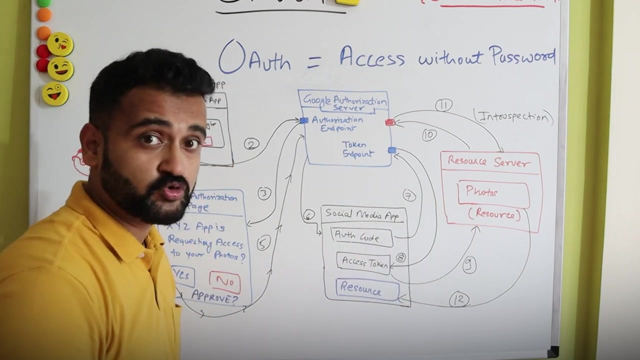 this media, social media application- is now authorized and have the access token to finally go to the actual resource server which is holding the user's photo at step nine, and then it will provide this particular access token and say, hey, I have got this token, can you give me the photos? but 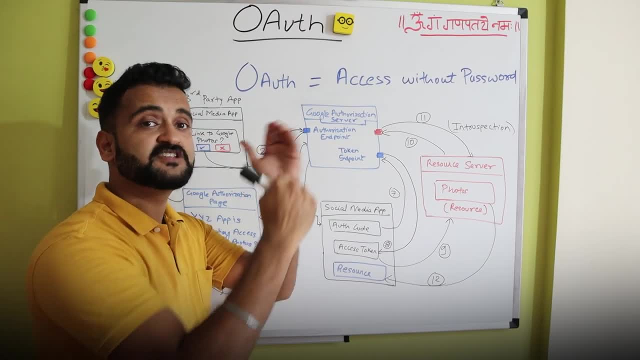 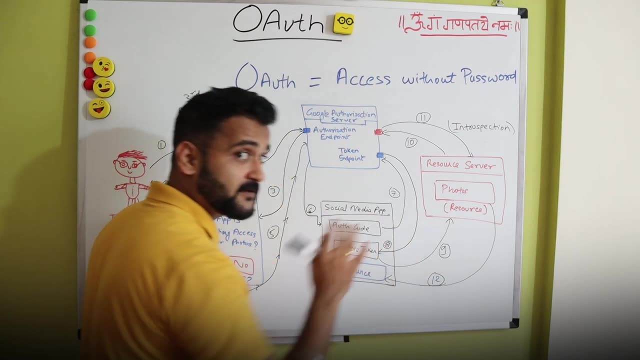 as I say, this whole scenario could be customized based on the security level, and I'm taking google, as you know, as the epitome of security for now. So now, even the resource server would not trust this token. even if the access token has come Now, the resource server will again go to this. 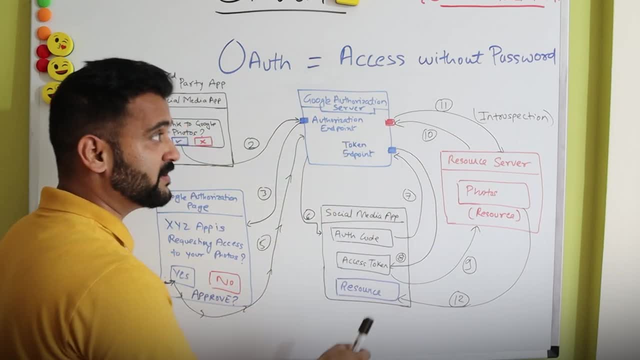 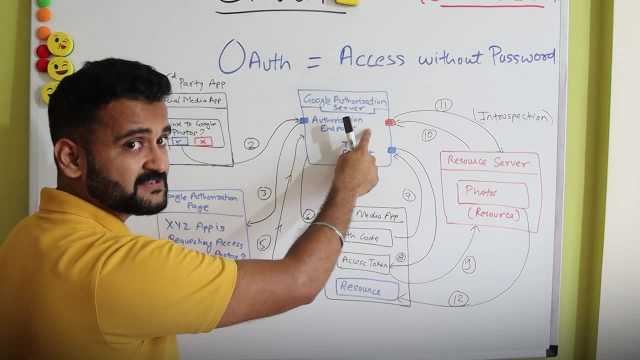 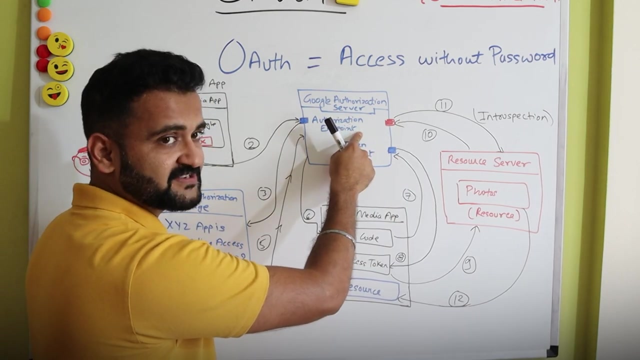 google authorization server. google resource server will go to google authorization server and this workflow is called as introspection, wherein the resource server will ask that whether this access token which this media app is providing is valid or not. So at 10 it will take this access token again to the authorization server and, in step 11, the authorization server. 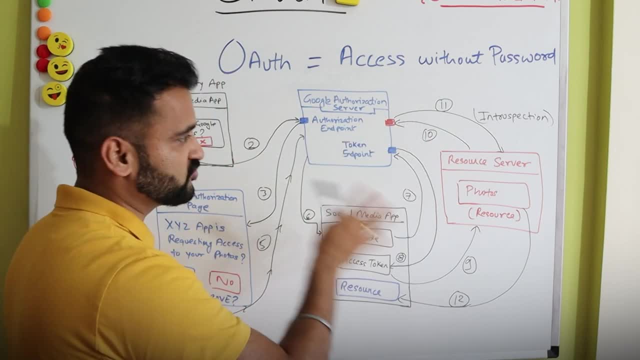 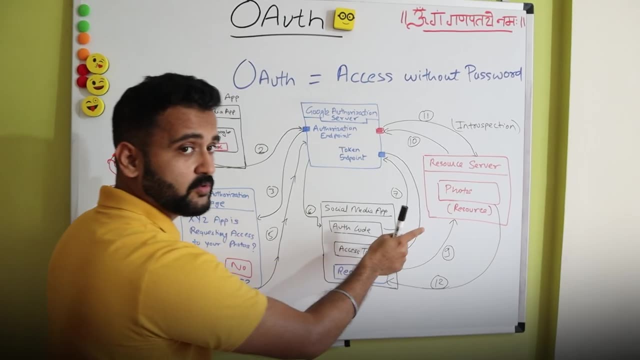 says: hey, don't worry, you know I have. I have myself given this access token, token so this application could be trusted. so at step 12, finally, after doing this workflow and after confirming the identity and the trust of this particular media app, at step 12, finally, 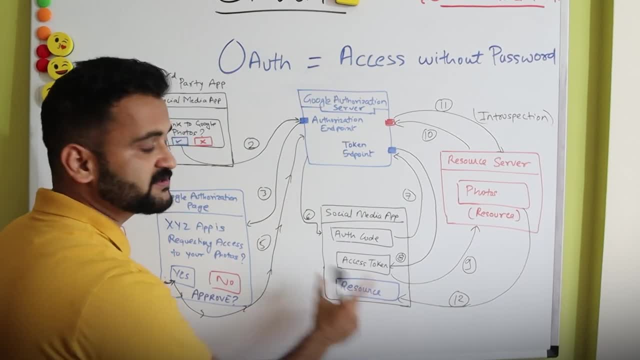 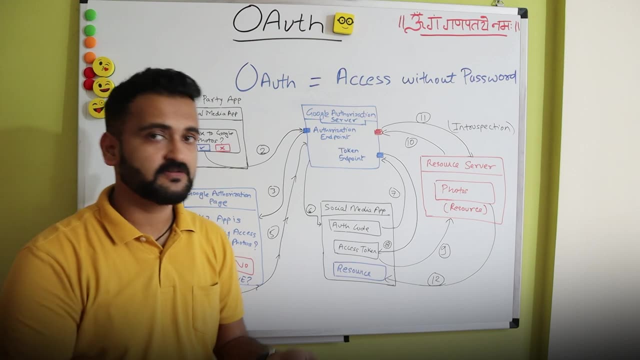 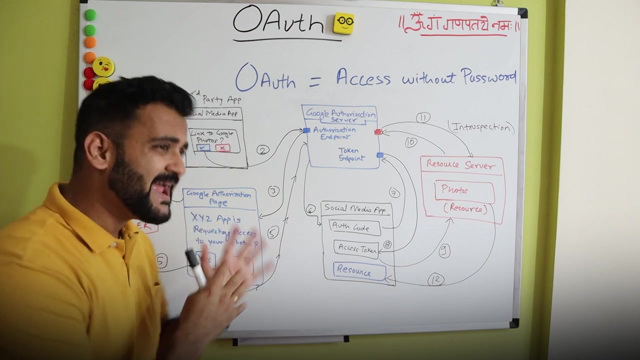 these photos are sent and as a resource to this particular social media application. so now this might look like a very lengthy workflow, but it happens in a split of um seconds or minutes. okay, this whole oauth protocol has been designed in a way where it is open standard, so anyone you know could use this oauth api and produce this whole workflow. 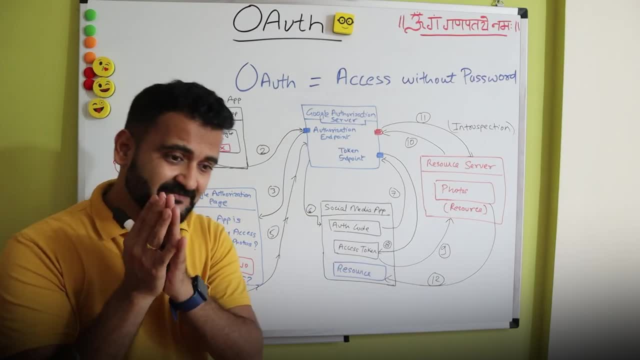 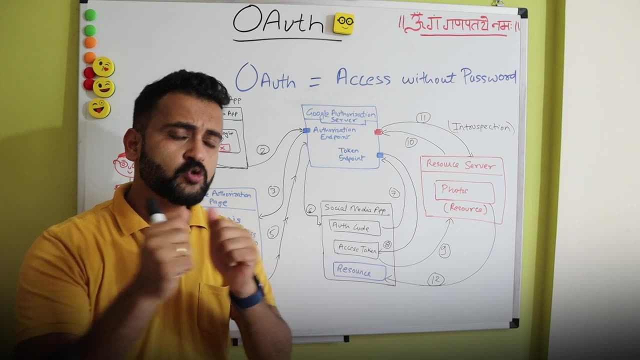 so i hope you now got this flow and how oauth works. and this is why oauth is so special, guys: because oauth democratizes your whole authorization system. you don't have to build your own. you could simply authenticate, authorize a user and get access to his or her resources. 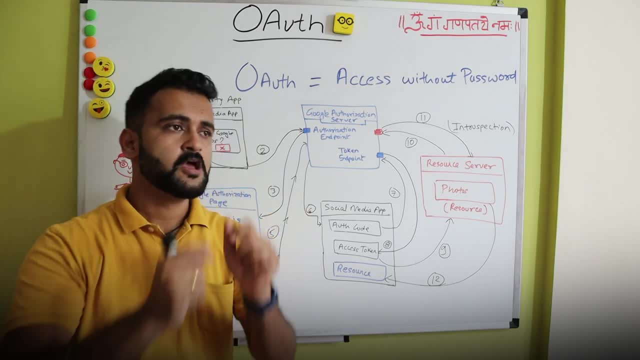 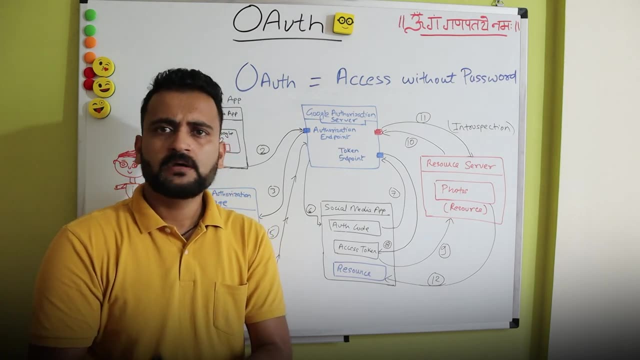 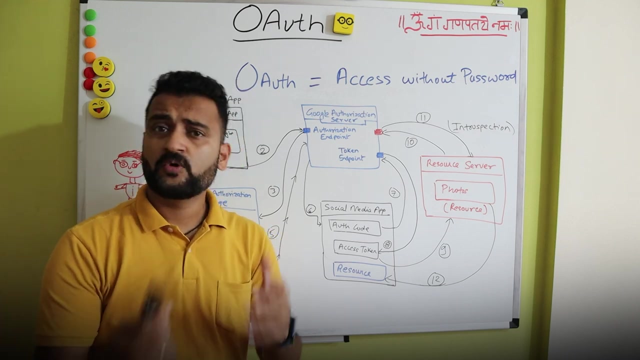 using oauth protocol because it's an open standard. that means, be it google, be it amazon, be it azure, anywhere you know any application. if you are building your own application, you can simply use oauth to get these resources or get authorization, and that's why nowadays we, as i said in the start, 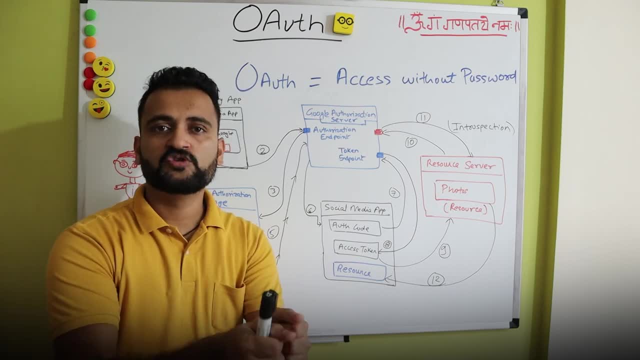 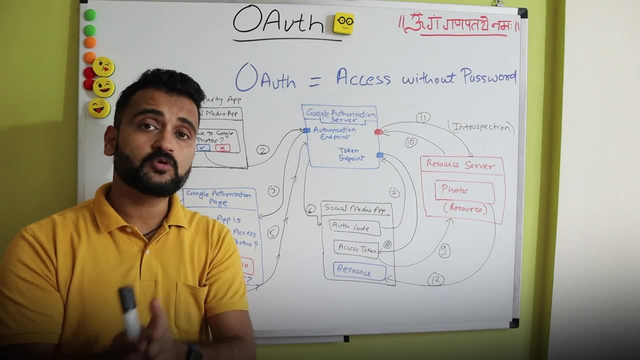 of the video. no one nowadays set up their own user id password on any of the apps, and that's the magic of oauth. so, friends, i hope you now know a bit about oauth and i hope this video was helpful. oauth and how exactly it works. just to reiterate, we have several components in oauth, starting from